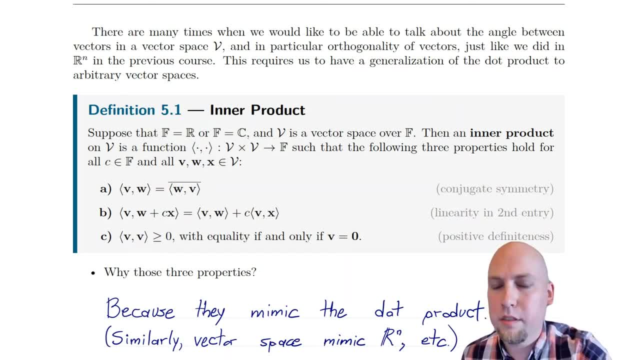 with an inner product. we're really going to need to be working with the real or complex numbers. Okay, I'll talk about why that it is in a minute. Okay, this does not work over arbitrary fields. you need real or complex numbers. Okay, then an inner product on that vector space. 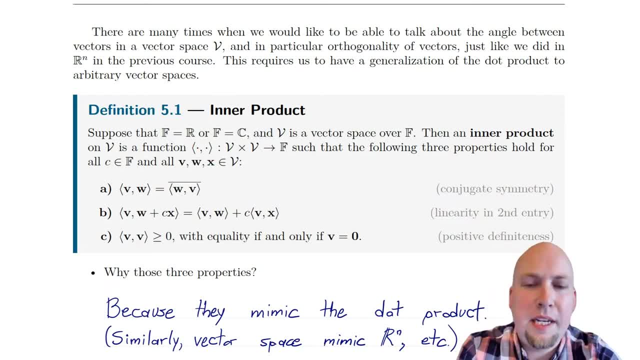 it's a function, And then this funky little notation here means. what this function does is it takes in two vectors from V and spits out a number. Okay, so there's V, cross V, that's the input, two copies of V and then F is the output, numbers are the output. 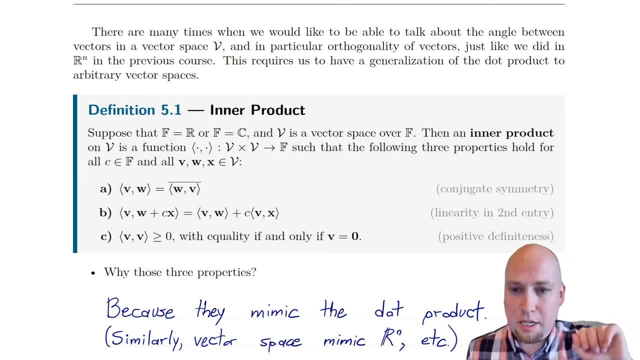 Okay, so, first off, your function has to take in two vectors, spit out a number, And also it's got to have a bunch of additional properties and in particular, these three additional properties down here. for it to be an inner product. The first property that it's got to have is what? 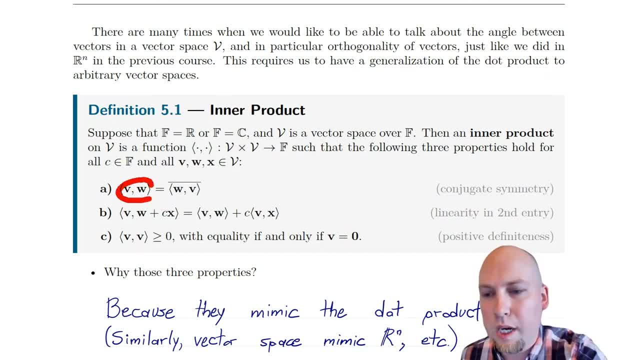 we call conjugate symmetry. Okay, and this just means if you swap the order of the input, so if you change V and W to W and V, then what happens is you pick up a complex conjugate over top of the inner product. Okay, 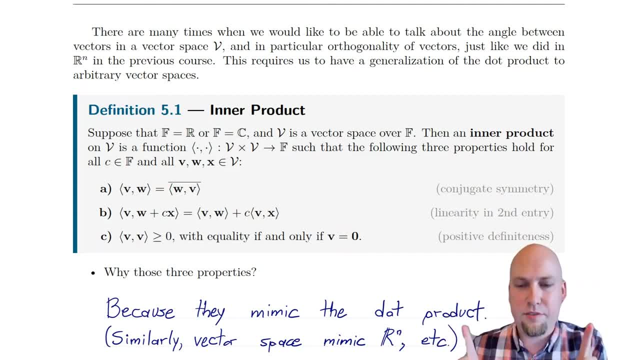 so it's not quite symmetric. you can't just swap the inputs freely, but you have to be careful. throw in a complex conjugate. if you swap the inputs, Okay, if the field that you're working over is the real numbers, then of course the complex conjugate does nothing. So in that case, 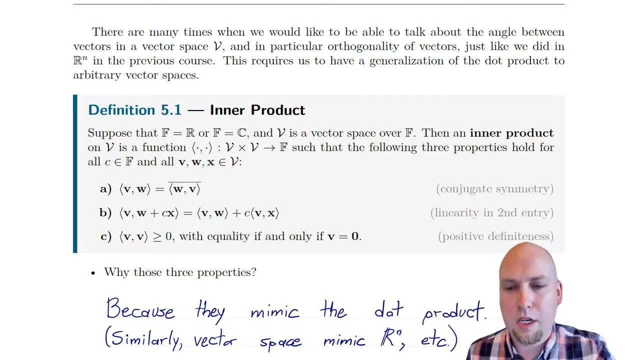 conjugate. symmetry is the same as symmetry, But in general, if you're working over complex numbers, don't forget the complex conjugate when you swap. Okay, the next property that we have is an inner product. it has to be linear in its second entry. In other words, if I leave the V fixed in the first, 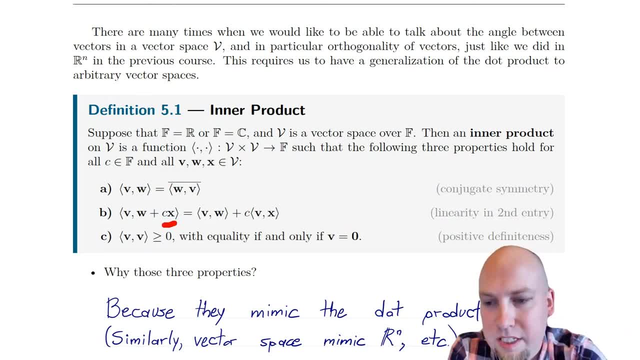 entry, it behaves kind of like a linear transformation in the second entry. right, We have W plus CX, splits up into a W plus CX. Okay, so it acts linear in the second entry of the inner product. And then the third and final property that you have to have is something that we call positive definiteness, And 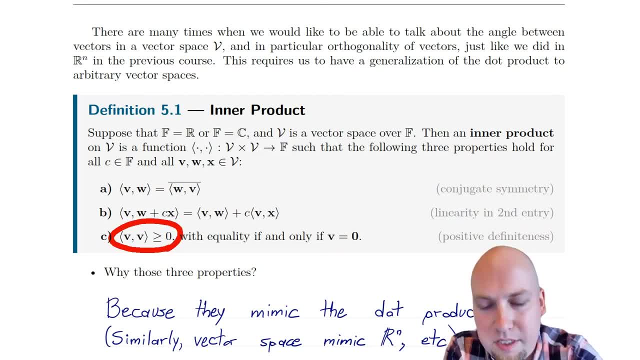 what this is is, if you plug in the same vector to both slots of the inner product, you always get a real number first off. even if you're working over the complex numbers, you get a real output from this, And not only a real number but a non negative real number. And even if you plug in the 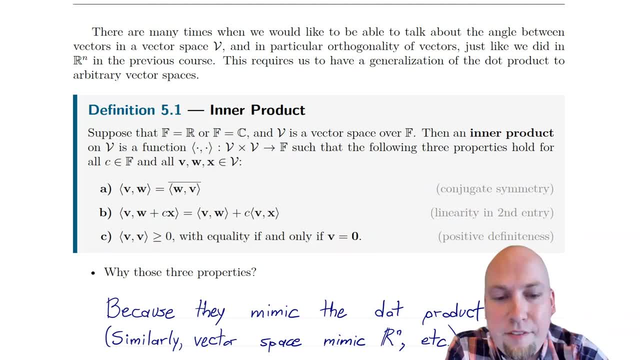 non negative real number, you get a real number. And even furthermore, the only way that you get zero is if you plug in the zero vector to both slots. Okay, so, in other words, if you plug in any non zero vector, you get some strictly positive real number here. Okay, so there's a lot to unpack in. 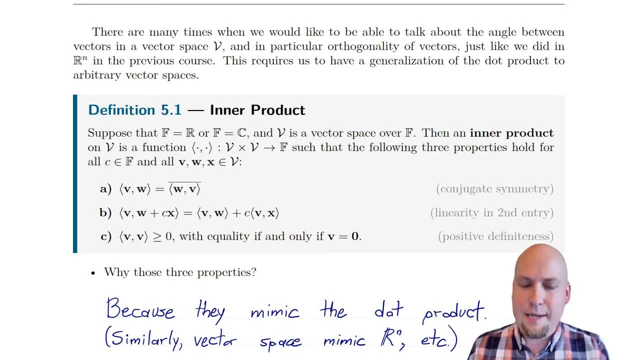 this definition a lot of. before we even going through some examples of this, Let's answer a couple questions that are probably floating in your head, like: why do we do these things? Like why is this defined this particular way? So, first off, I suppose we're going to have to think about: 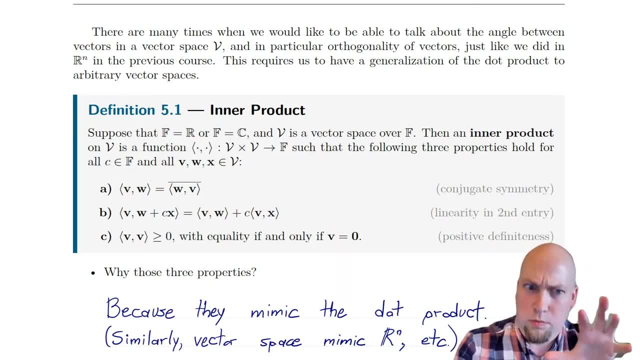 why we need the real or complex numbers, Like: why is that? And that is because in general fields, like if you have some other number field other than real or complex numbers, you might not have an order. you might not have an order of those numbers right, You might not be able to say: 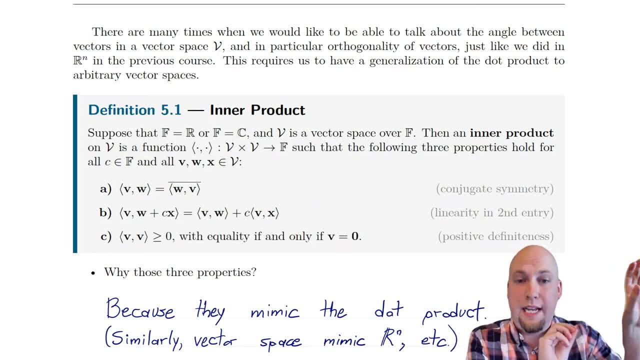 hey, this number is bigger than this number, even than the complex numbers. actually, we don't have sort of a natural field ordering Okay, but we sort of need one right for this property C here to make sense, we need to be able to talk about the output of this function, which is in the 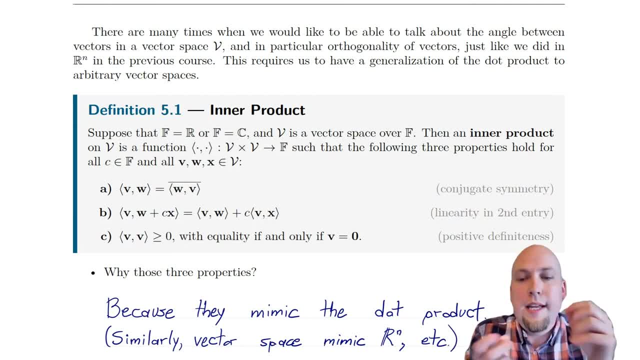 field being bigger than or equal to zero. Okay, so the reason that this works with the real numbers is because there's a nice ordering on the real numbers. The reason that it works with the complex numbers is because this quantity here, even if you allow complex outputs in general whenever you- 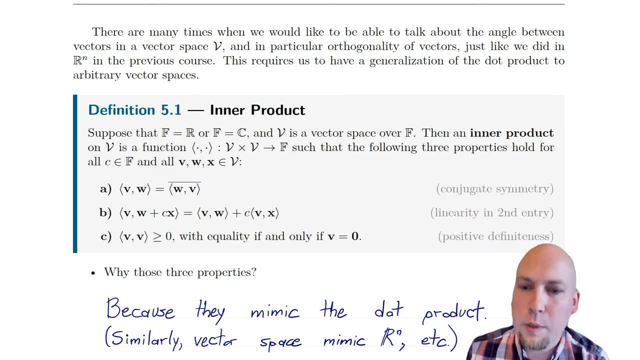 plug in the same input to both slots, you always end up getting a real number anyway. Okay, and that follows from conjugate symmetry. actually okay, because if you swap the inputs, nothing changes, but you also pick up a complex conjugate. In other words v. inner product. v is 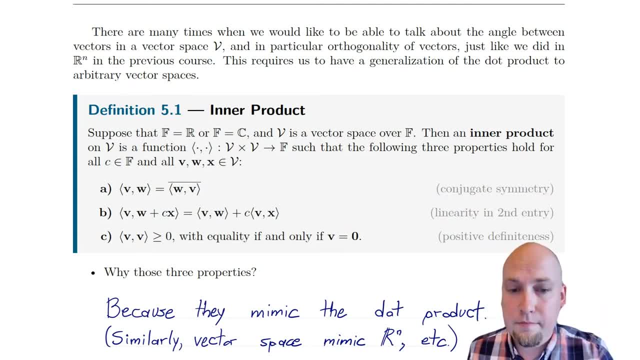 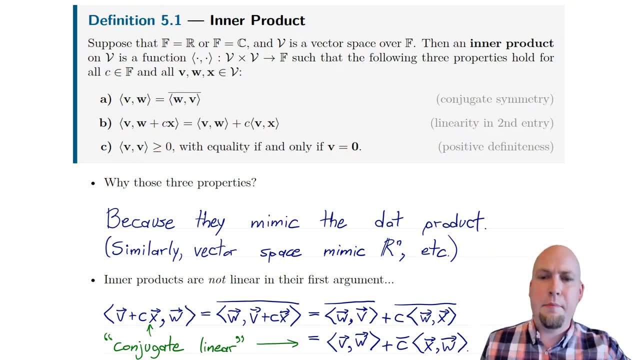 always going to be real, because it equals its own complex conjugate. Okay, another question that pops up when you look at this definition is: well, why these three properties here? Why properties A, B and C? And, of course, the reason for those three properties is because we want this to mimic. 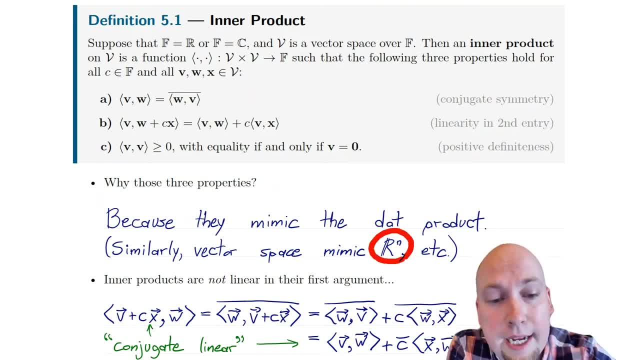 the dot product on Rn right And if you go back to introductory linear algebra right after you saw the dot product, you would have seen properties that looked exactly like this, except written using dot product notation rather than inner product notation. 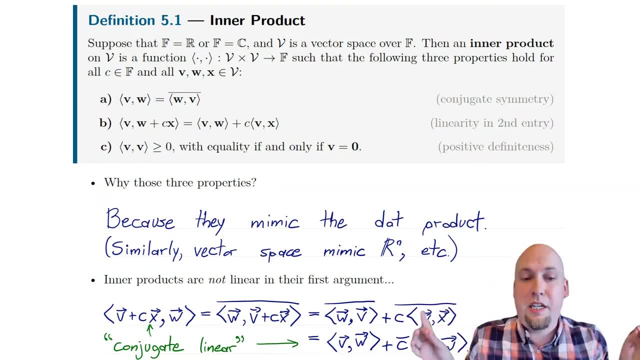 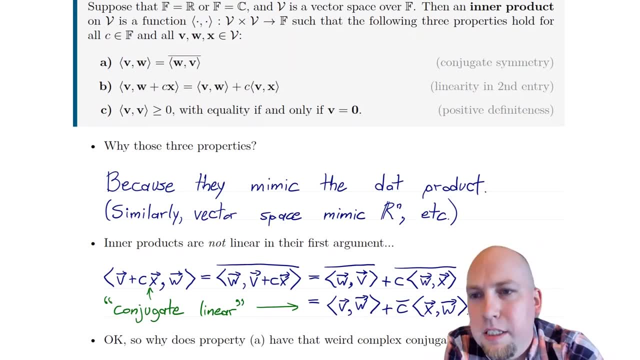 Okay, so it's just like vector spaces. We define vector spaces to mimic Rn, while we define inner products to mimic the dot product. Okay, one thing that you have to be a little bit careful of is property B. here, Inner products. they're linear in the second entry. They are not quite linear in. 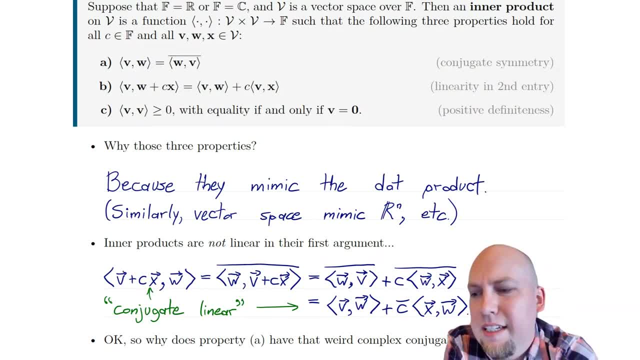 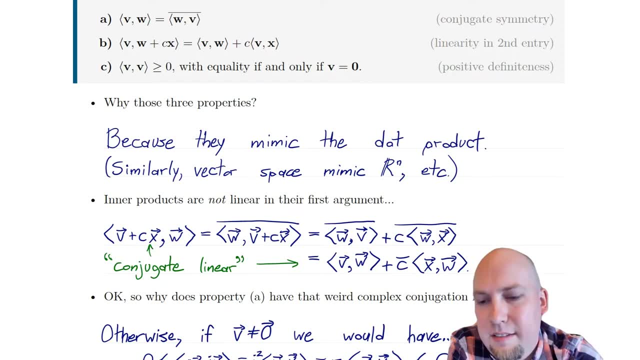 the first entry. You can use conjugate symmetry to show that they're kind of linear in the first entry, but not quite okay. So if you use conjugate symmetry to try to figure out what happens if you have a linear combination in that first entry, there, well, you swap things with conjugate. 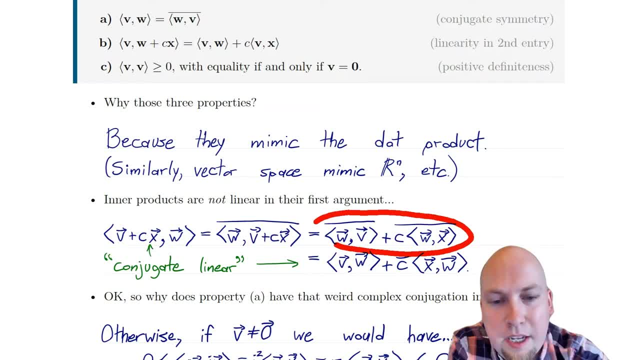 symmetry, property A, and then you can split things apart using property B, linearity in the second entry. And then, hey, these are all just numbers and I can pull the complex conjugate onto each of the inner products individually And when I swap them back, when I swap this inner product, 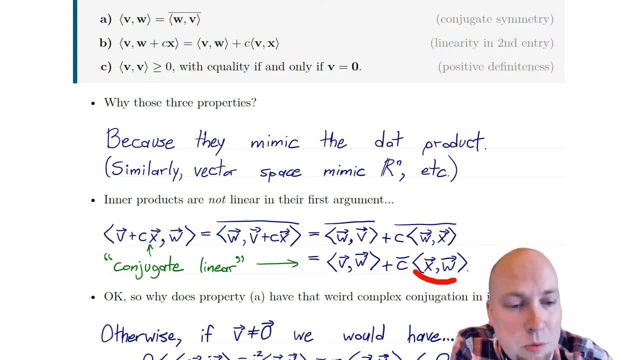 back, the complex conjugate goes away. And similarly, when I swap this one back, the complex conjugate goes away. But one complex conjugate that never goes away is the one over the scalar here. Okay, so what happens is if you have V plus CX, inner product with W, you get V with W plus complex. 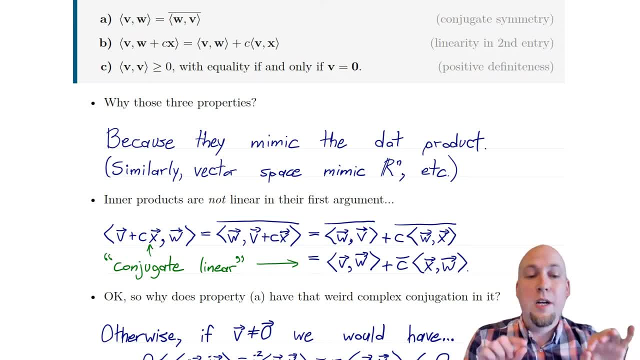 conjugate of CX with W. okay, So it's almost linear. except you picked up complex conjugates over top of scalars, So it's what we call conjugate linear. okay, So you can sort of split up linear combinations in the second entry and you can split up linear combinations in the first entry. 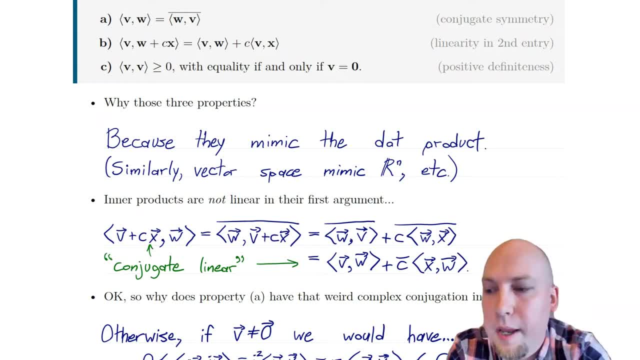 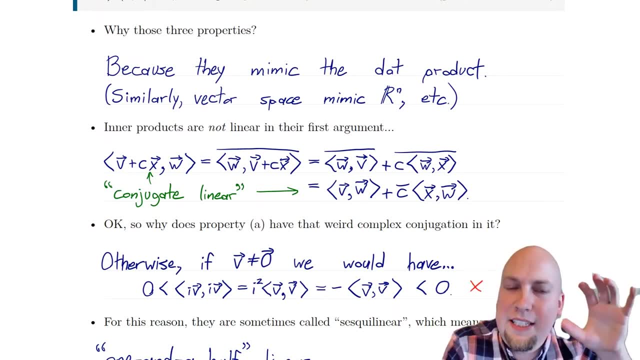 but only as long as you remember to put complex conjugates over your scalars. Okay, Now let's look back here. I said that we introduced these three properties so that these inner products, they would mimic the dot product. But wait a second, I mean. 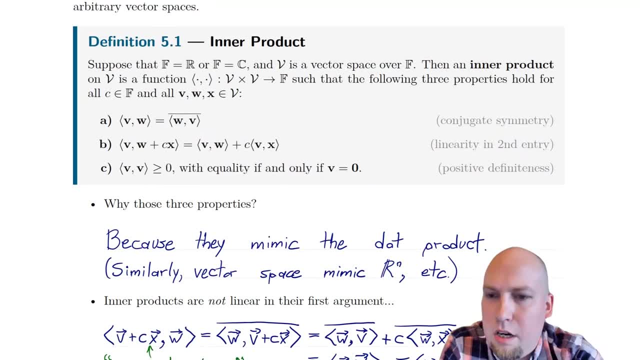 in the original dot product, like the original dot product on RN is just symmetric right V dot W is the same as W dot V. So why did we throw this weird complex conjugate over top here? Where does that come from? Okay, Well, think about what would happen if we didn't have that there. Well, plug in. 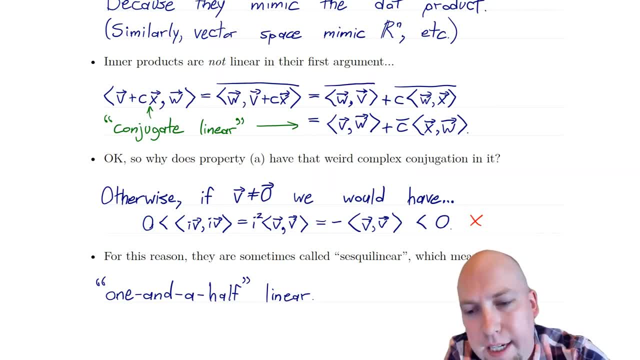 any non-zero vector into your inner product then and what you're going to get is: hey, inner product of V is the same as W dot W. So what do you do? You plug in any non-zero vector into a non-zero vector. with non-zero vector, That's got to be bigger than zero, Okay, So I just took. 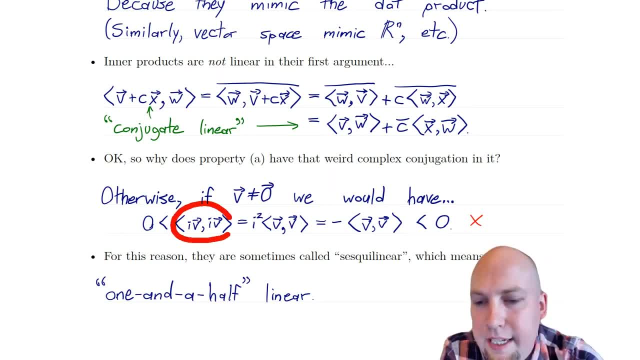 whatever non-zero vector I like and multiplied it by I. And then here I use property C to see that this is bigger than zero, strictly bigger than zero, Okay. But now if property A didn't have that weird complex conjugate in it, I could just pull each of these scalars out and I wouldn't need. 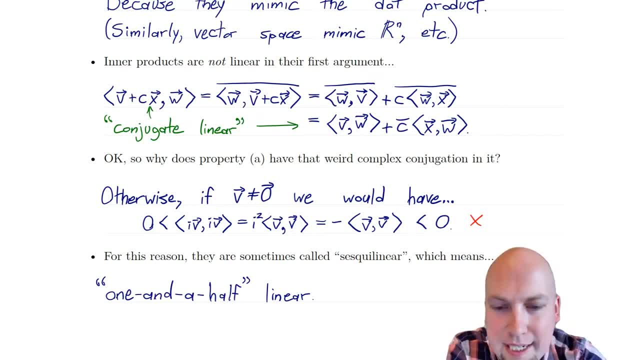 to throw complex conjugates over either of them, So I'd end up getting an I squared over out in front, rather than an I and a minus I. So I just get I squared out in front, and I squared, of course, just equals minus one. So I get a minus one out in front. But now I'm left here with minus the. 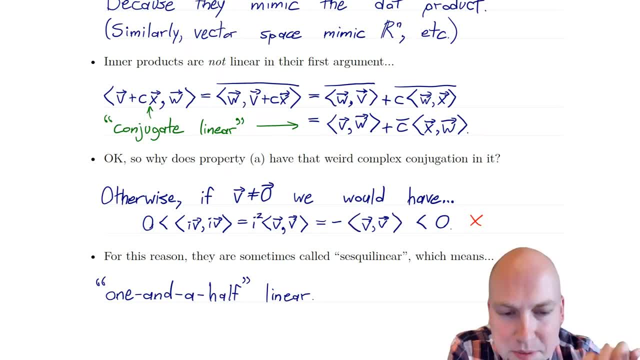 inner product of V with itself, And because this inner product of V with itself must be strictly positive, negative of it must be strictly negative. So what we found here is that zero is strictly less than some junk which is strictly less than zero. So zero is strictly less than itself, And 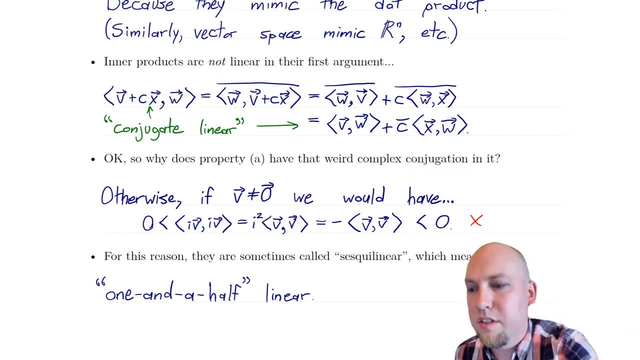 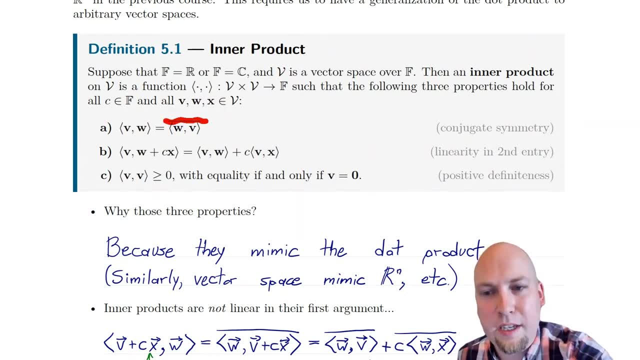 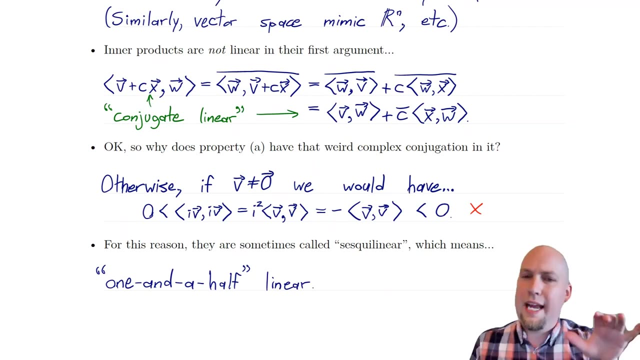 that, of course, cannot happen. Okay, So there's no way to define a function that actually has all of these properties, But without the complex conjugate there. Okay, You need the complex conjugate to actually find functions like this. Okay, And because we only have this weird conjugate linearity in the first, 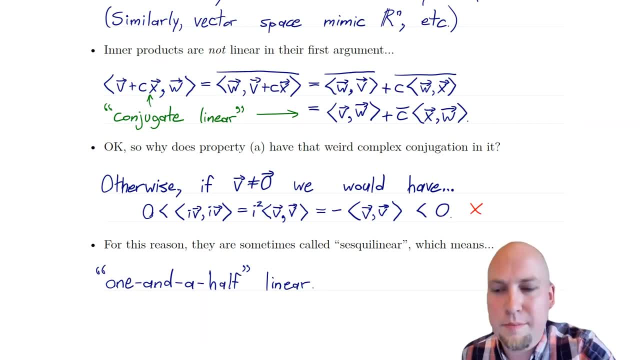 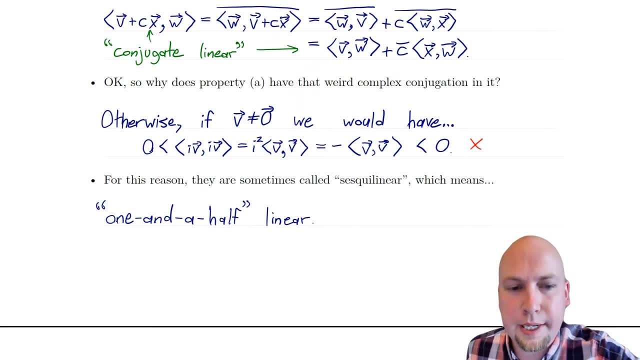 property. we sometimes call these functions sesquilinear, which just means one and a half linear. You know it's linear in the second entry and you know it's sort of half linear, It's kind of linear in the first entry. Okay, So let's go through a bunch of examples of inner products. 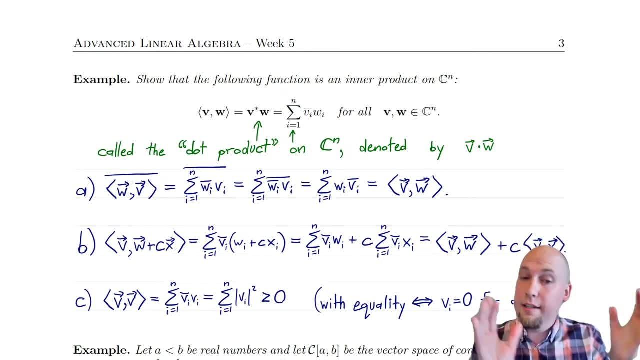 and various vector spaces that we've been working with. We, of course, have already seen an inner product on Rn Right, Just the dot product. So that's just an exercise to go through to check, maybe convince yourself that, yeah, the dot product on Rn really is an inner product. It satisfies those three. 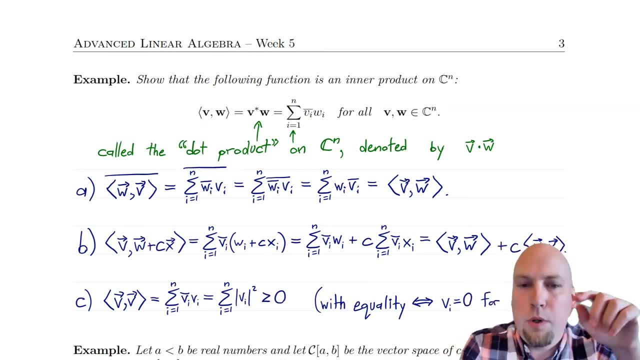 properties from that definition up above All right. Well, a very similar inner product exists on the vector space Cn. So complex numbers, but n of them in a list. Okay, And this is actually also called the dot product. Okay, It's called the dot product on Cn or the complex dot product. 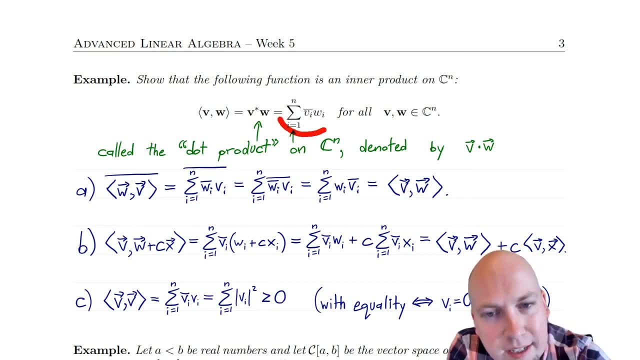 And what it is is? well, it's just. you do the same thing as in the dot product: You take all the entries of v and w and you multiply them together and you add them up, except you throw a complex conjugate over top of the entries. 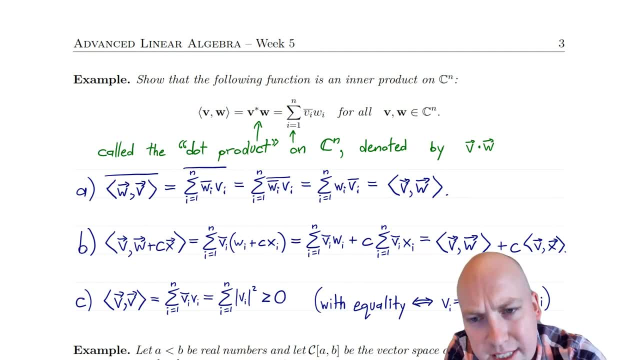 in the first vector. Okay, And maybe we haven't seen this notation before yet- This v star- here I'm thinking of v as a column vector. The star means transpose it, So turn it into a row vector and also put a complex conjugate on every entry. Okay, So this is just a different way. 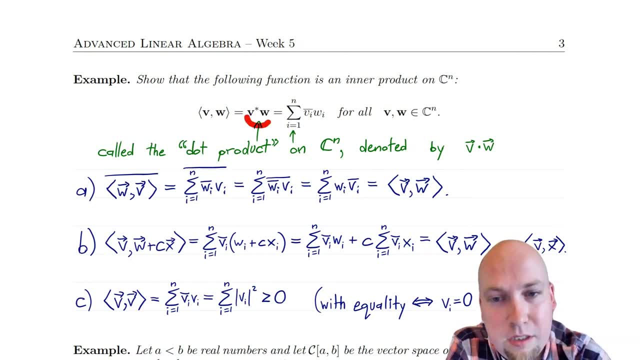 of writing this exact same formula here, Okay. So if you don't know, if you don't like the like that, just remember this, it's the same thing. Okay. So let's show that this actually is an inner product. Let's show that this complex dot product really is an inner product And the 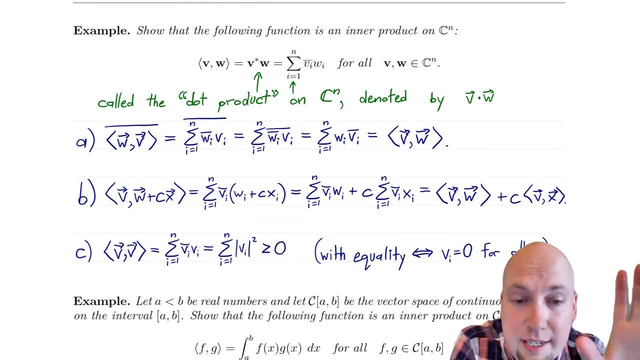 way you do that is, you check the three defining properties in the definition of an inner product. So the first property to check is that if you swap the order of the two vectors in an inner product and put complex conjugate over top, then you'd better get the same thing as just the original. 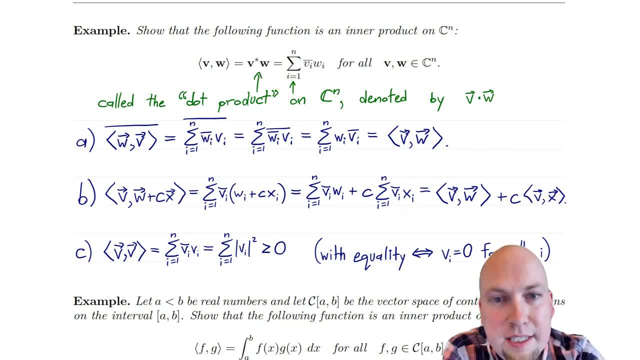 inner product itself. Okay, So let's just check using this formula for the inner product. Okay, So we've got the inner product v. Well, that's just the sum of the wi's with a complex conjugate over them, because they're the first vector in the inner product times the vi's, and then you add: 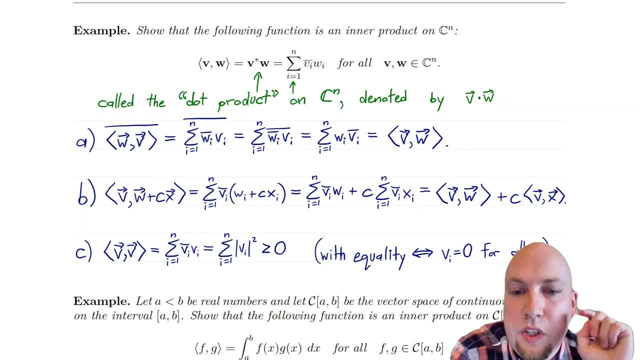 them up and there's this complex conjugate here just over top of everything. Okay, And if you have a complex conjugate over a sum, you can just put that complex conjugate over top of every entry in the sum And then over on the left here we've got complex conjugate of a product of two numbers. 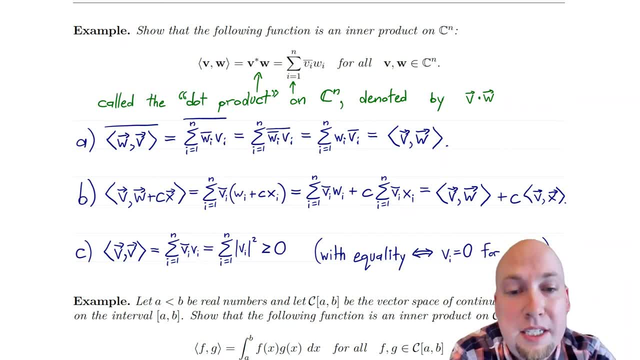 Again complex conjugate. it splits up over products, so it's a complex conjugate of each of them individually. And then the wi's have a double complex conjugate over them, So you're over top of them. and complex conjugating twice just gets you back to where you started. So wi. 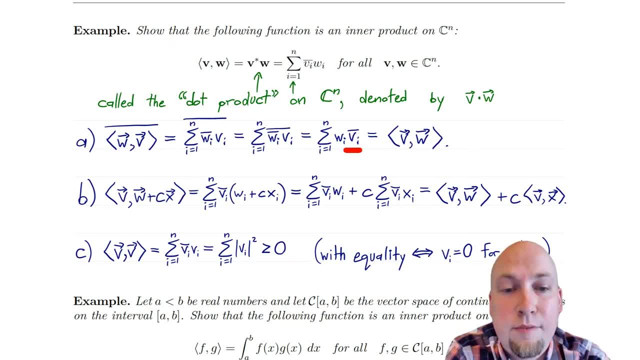 conjugate to conjugate just equals wi itself. So we're just left with this sum here, And if you just swap the order of the terms here, so you have vi bar times wi. you see this is exactly the complex dot product itself. It's the inner product that we started with, So yeah, 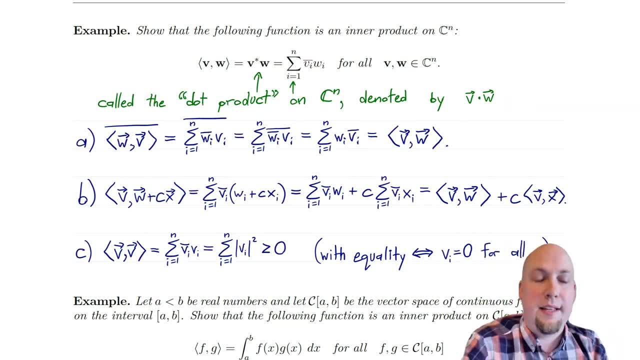 this left-hand side does equal the right-hand side, So we're happy with that. Okay, Property a is satisfied. Property b: you just plug in the linear combination into the second entry and then you plug all that back into this definition of the complex dot product. So you: 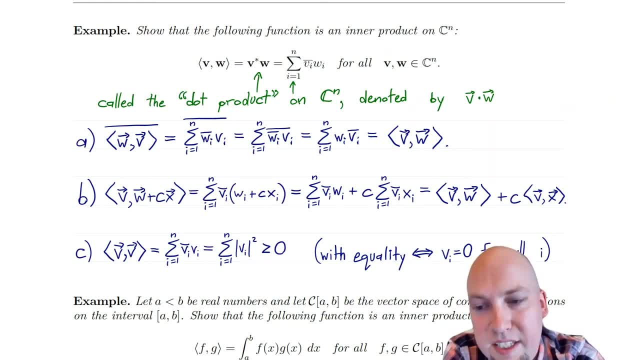 got vi bars, and then the ith entry of the second vector. Well, the ith entry of the second vector is wi plus cxi. And then: well, those are all just complex numbers, so you can use your usual arithmetic rules with complex numbers. right, This is a sum of a product, and then there's a sum here. 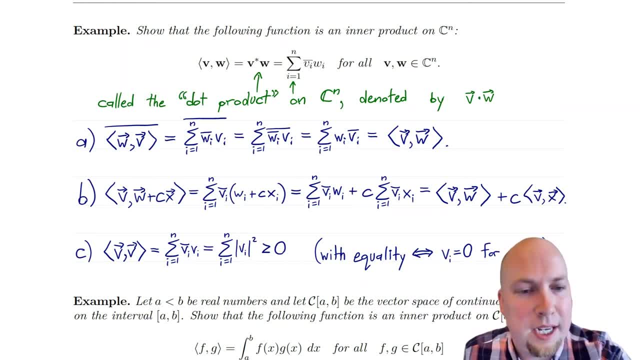 Just distribute things, okay. So you get a sum of vi bars wi's and then this sum over here, and those are just the individual dot product. Okay, So nothing fancy happens there. It's just your usual arithmetic rules, just sort of n times because there are n terms in the sum. Okay, And then finally property c. 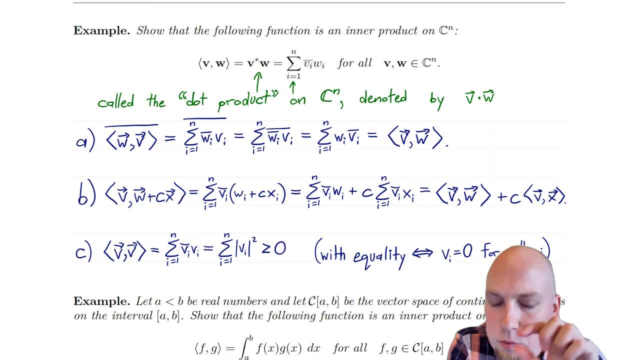 we've got to show that the inner product of v with itself is bigger than or equal to zero And, furthermore, the only vector that gives you zero inner product with itself is the zero vector. All right, So the way that we do this, again plug into the definition, right, It's just my w's are. 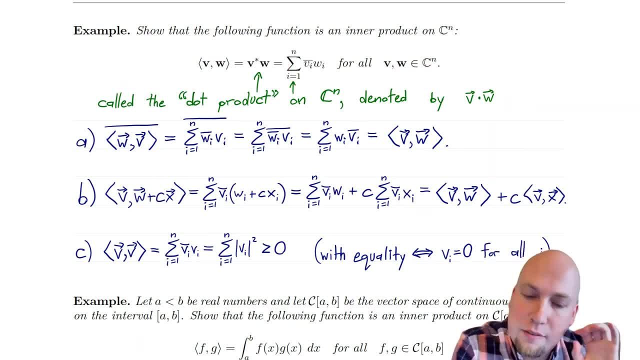 v's now. So I get sum of vi bar vi. and one of the nice properties about the complex conjugate is the complex conjugate is the complex conjugate. So the complex conjugate is the complex conjugate of a number times itself just equals the length or magnitude of that complex number squared. 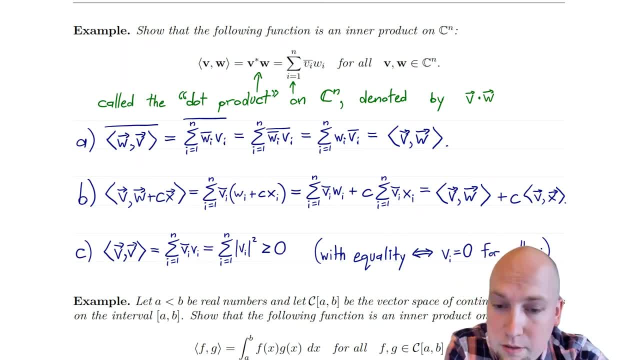 Okay, So you've got a length squared that's bigger than or equal to zero, and then plus a whole bunch of other length squareds also bigger than or equal to zero. So the whole thing is bigger than or equal to zero And, furthermore, the only way that this sum can equal zero is if each of these lengths 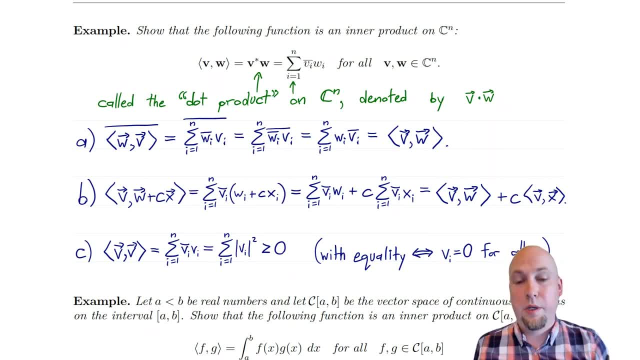 equals zero. In other words, each vi has to equal zero. In other words, v must be the zero vector right. Each of its entries must be zero for its equal to zero. So that's what we're going to do, All right, So that's the whole thing That shows that, yes, this function up here. 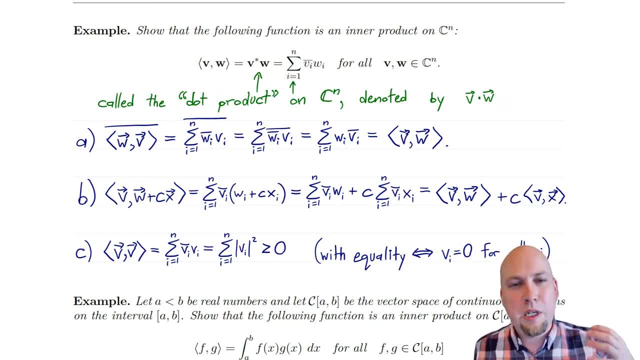 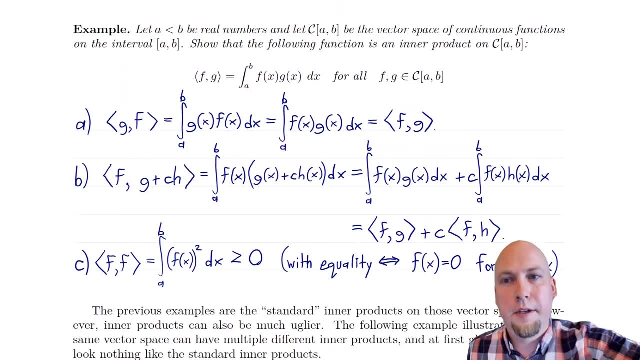 this complex dot product really is an inner product And we call it the standard inner product on Cn, just like we think of the dot product on Rn as the standard inner product on Rn. Okay, But there are lots of other inner products as well, though We'll see more of them as we go. 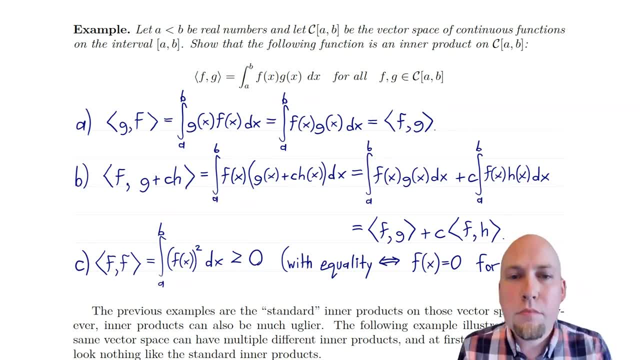 but it's good to be really familiar with these standard examples. Okay, So let's go through another example on a slightly more exotic vector space. This time we're going to be working with the vector space. We use a curly C here to denote set of continuous functions And the set of 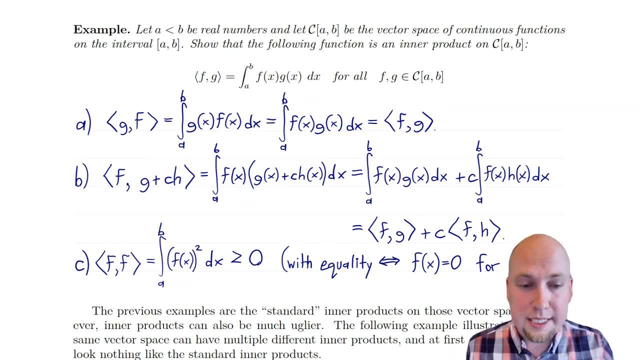 continuous function is a vector space- Okay, We haven't worked through it explicitly in these lecture videos, but it is Okay. And this square bracket A to B: that means I'm only considering the continuous functions on the real interval from A to B, So I'm not considering how they. 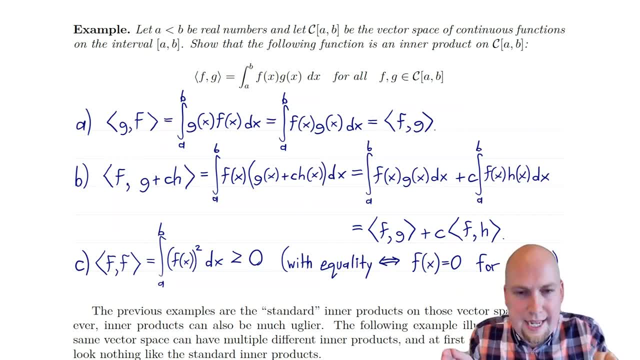 behave on the entire real line. I'm only considering how they behave on that interval from A to B. All right, So on this vector space here, let's show that this function here is an inner product. Let's show that if I integrate the 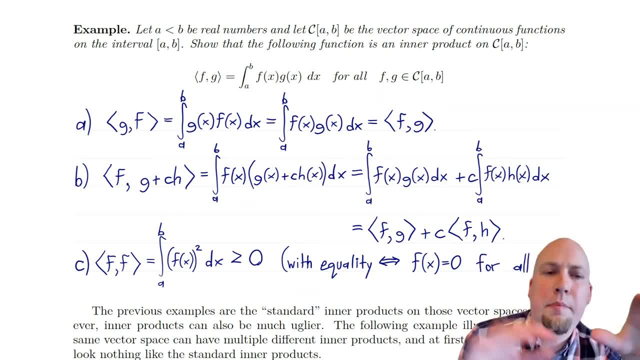 product of those two functions. from A to B, I get an inner product. And before we go through why this is the case, sort of rigorously, by checking those three properties, let's think sort of intuitively about why this feels like an inner product. Okay, The only examples that we've seen. 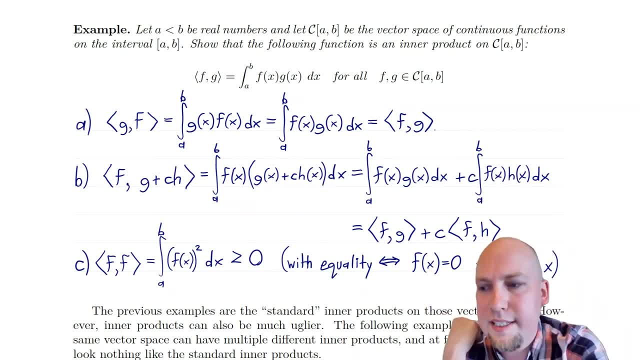 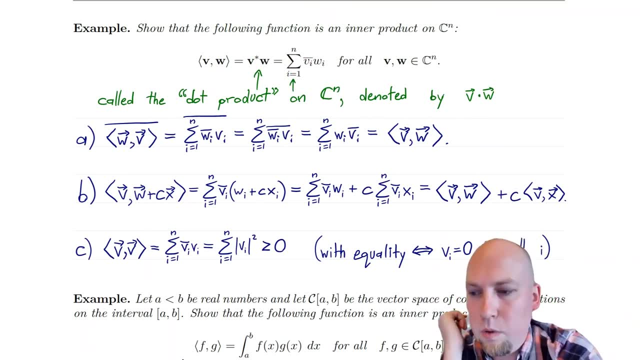 so far are the dot product. And for the dot products, what you do is you take one of the vectors and you multiply it by the other one, but just sort of entry-wise, and then you add them up. Well, what are we doing in this example? here Again, we're multiplying. 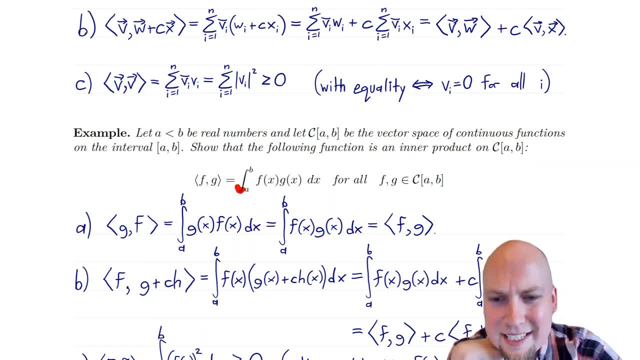 the two functions together entry-wise And then in a sense we're sort of adding them up. It's just the function version of adding right. We sort of have infinitely many points to add up. Roughly speaking, the way you do that is via an integral. So again, like this should feel. 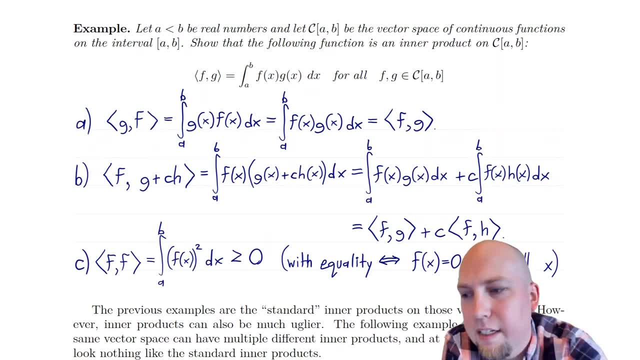 sort of like the dot product. Okay, So it feels like an inner product, All right, But how do we actually prove that properly? Well, again, just go back to the definition of everything You got to check these three properties. I have to check conjugate. 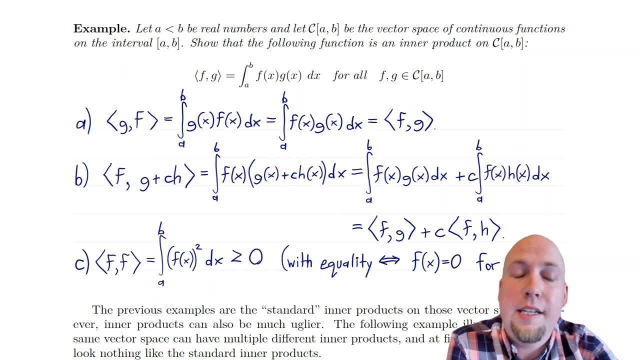 symmetry, but hey, it's a real vector space, So it's just symmetry. Is the inner product of G with F the same as the inner product of F with G? And yeah, it's just. hey, one of them's an integral. 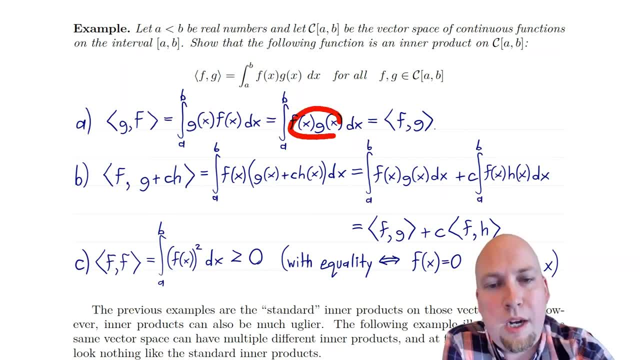 and the other one's an integral and they just have the order of the function swapped. So in other words, you're just multiplying real numbers in the opposite order. So yeah, that's true, All right. Property B: can I sort of take out linear combinations in the second entry, Is it? 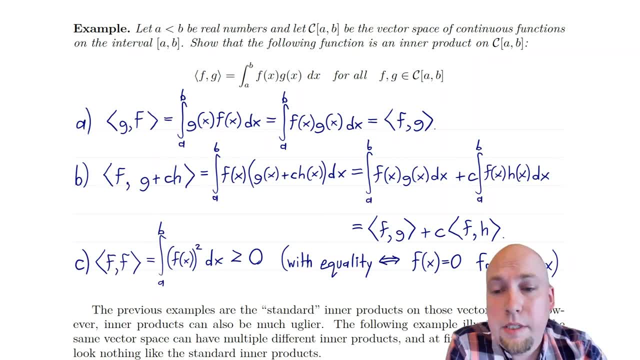 linear in that second entry. And again, yeah, this just follows from properties of real numbers and integrals right here. Okay, So this is the integral that we get if we plug this stuff into the two slots of the inner product here. Okay, 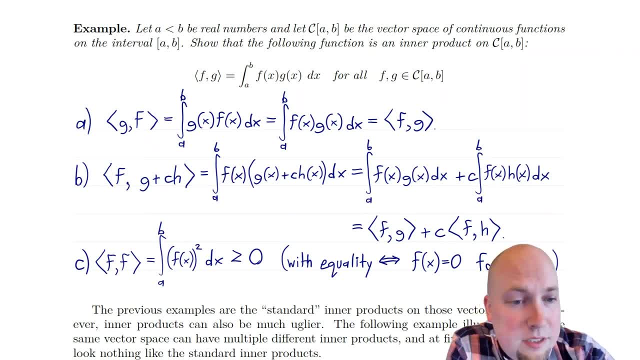 And then, hey again, FX times GX. So it gives me that first term. And then I distribute, I get a C times F times H, and I get that And I can split it up into two integrals, because you can do that with integrals. If you have an integral of a sum, that's a sum of 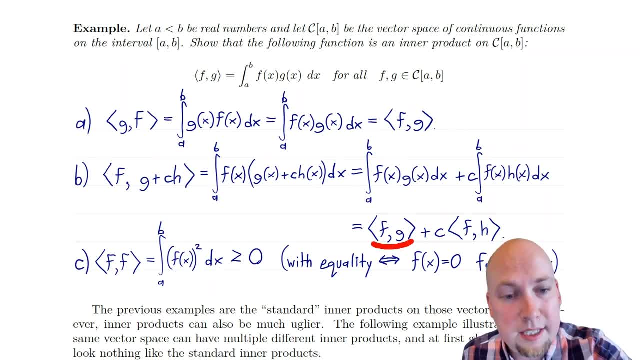 integrals, Okay. And then, hey, this is one inner product, that's F with G, and then this is C times F with H. So again, nothing fancy happening there. Okay, Property C is slightly more interesting because property C, okay, inner product of F with F, that's the integral. 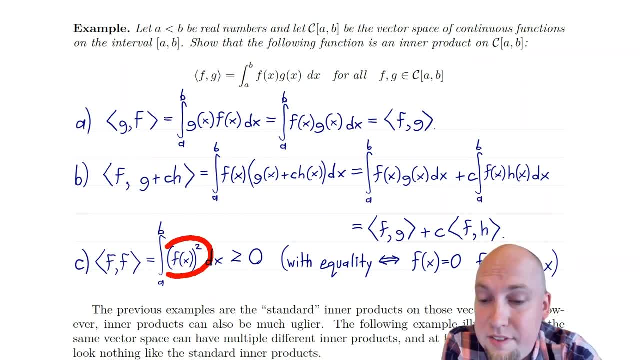 of F times F. So in other words, it's the integral of F squared. Okay, Great, That's bigger than or equal to zero, because each of these numbers is bigger than or equal to zero. And then I'm integrating that function. So you're integrating a function whose graph is above. 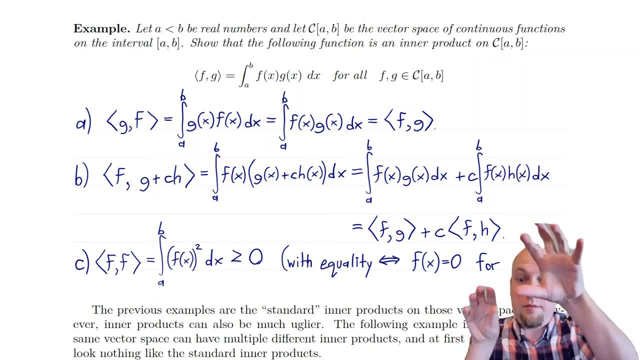 the X axis, right? Well, that area under the graph is going to be bigger than or equal to zero, right? If the function never dips below the X axis, its integral can't be negative. You're measuring an area that's above the X axis. So, yeah, this is bigger than or equal to zero. But furthermore, 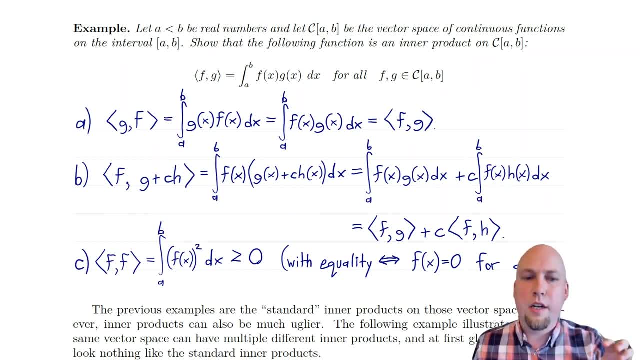 we need equality to happen if, and only if, we're talking about the zero function. Okay, And that is true, because, well, sort of roughly speaking, think about like, how could this equal zero? Well, each of these things, they would have to equal zero. 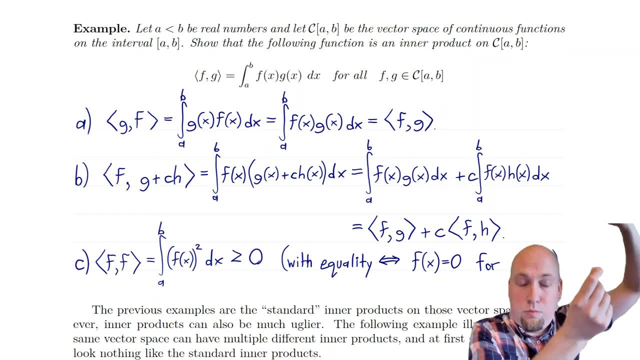 for the whole integral to equal zero, right? Because again, you're adding up, roughly speaking, all of these pieces above the axis. Okay, So the only way that this whole integral could be zero is if each of these is equal to zero, In other words, if F of X equals. 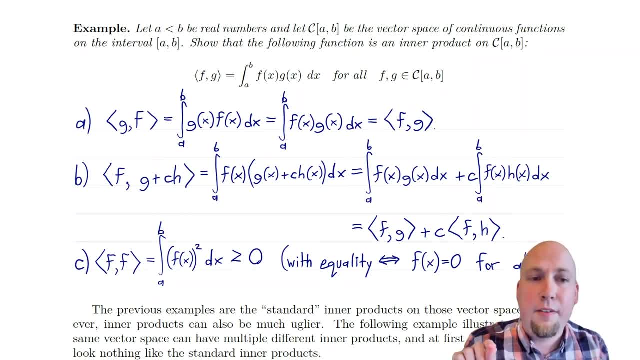 zero for all X, Except. you have to be a little bit careful there. I lied a little bit there. This is why we need to work with the vector space of continuous functions. Okay, This is why we're only considering continuous functions. Everything that I just said there is wrong. 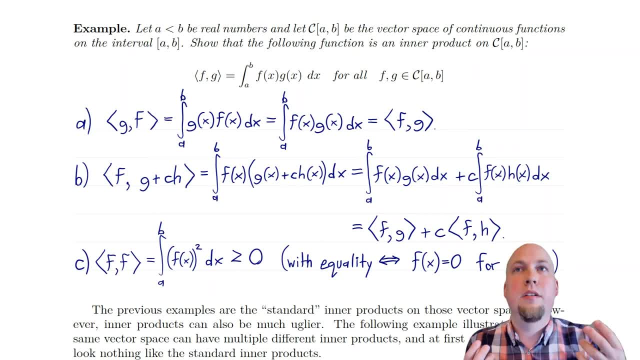 if you go outside the realm of continuous functions, Because you can have annoying little things like a function that's zero everywhere except hey, it takes on a value of one at three. When you plug in X equals three, its value is up at one, but everywhere else it's down at zero. 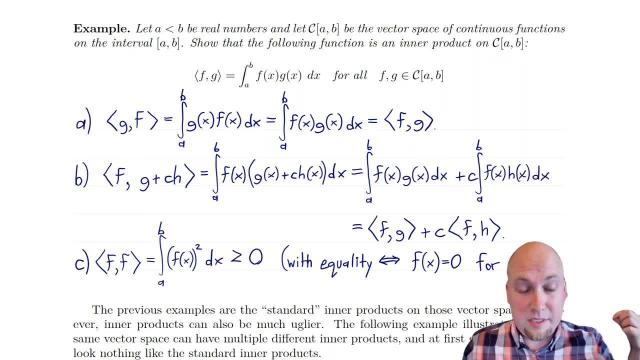 That function's integral integrable and it has integral equal to zero. basically because there's- even though at one spot it's up, at one, it's not up at one enough to actually affect the integral, but it's not the zero function. Okay, So we really do need to be working with continuous functions. 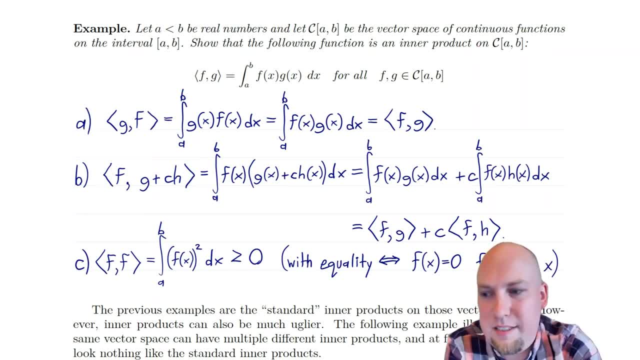 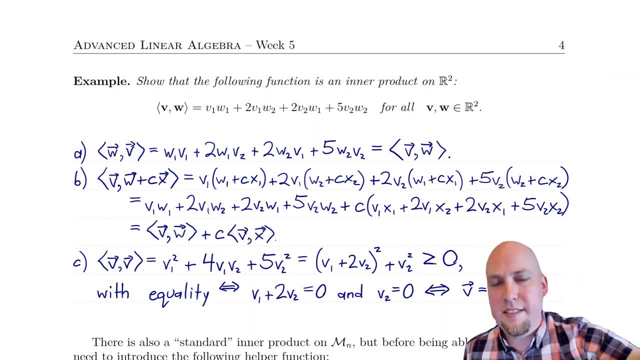 here for this to be an inner product, Okay, Otherwise things get a little bit murkier. All right, So those examples, those are all standard inner products on the spaces that they act on. Okay, But there are also lots of non-standard inner products as well. So let's. 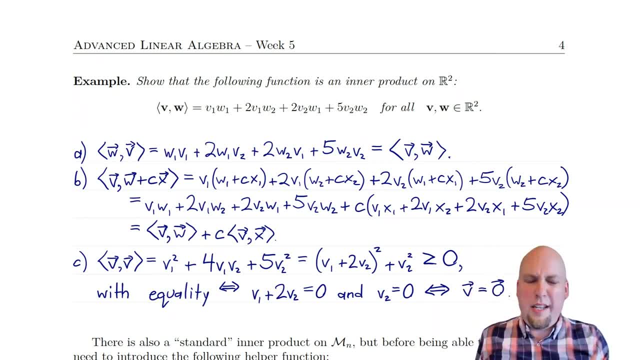 look at a non-standard inner product on R2.. Okay, By non-standard I just mean sort of not a usual one, not one that's going to come up over and, over and over again, or anything like that. Okay, So let's try to convince ourselves that this weird. 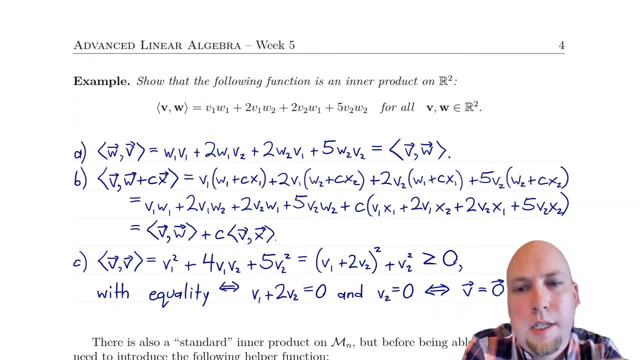 ugly function is an inner product on R2.. Okay. So again, it's kind of like the dot product, except we've got weird weights in there. We've sort of got cross terms as well. It's not just V1, W1 plus V2, W2. It's sort of nastier than that, but it is an inner product, Okay. So. 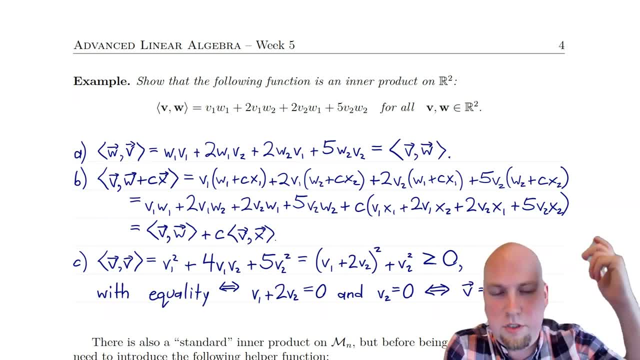 properties A and B. maybe I won't go through those because they're sort of just straightforward. You just swap everything around And because these two coefficients here are the same, everything works out Okay. And similarly with sort of pulling linear combinations of the second. 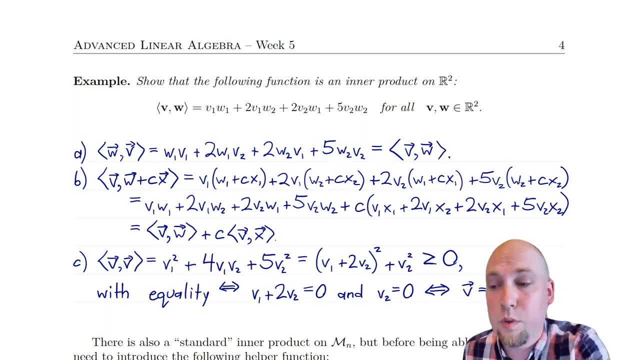 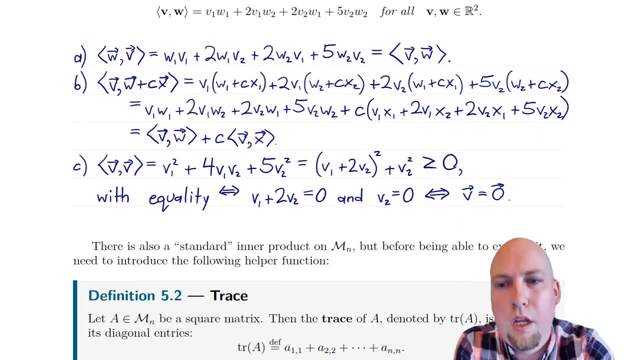 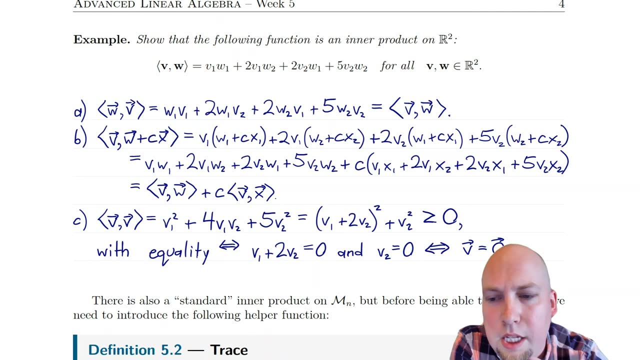 entry. it's just use your usual laws of arithmetic on R2.. Sorry on R. Okay, They're just real numbers that you're adding up here. Okay, The interesting property is property C. Is this function non-negative if I plug the same vector into the two slots? 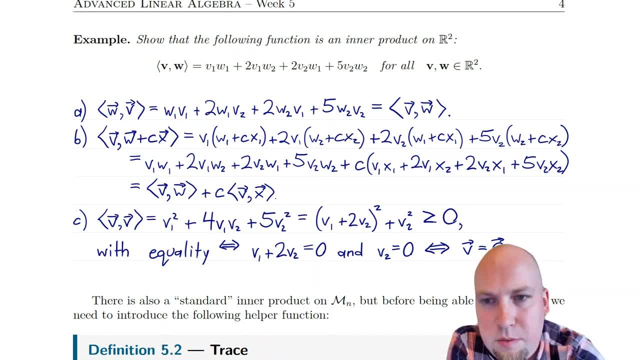 Okay. So what do I get if I plug the same vector into the two slots? Well, here I'm going to get a V1 times V1, in other words, V1 squared Over. here I'm going to get five V2 times V2, in other words, five V2 squared, And then each of these cross terms is going to: 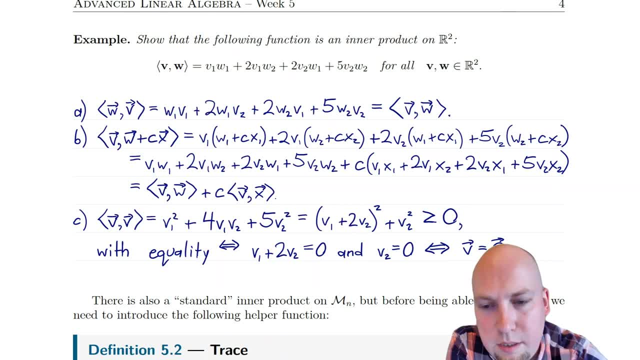 give me two times V1 times V2.. Okay, So I'm going to get four times V1 times V2 as my overall cross term from these two terms. Okay, That is not obviously bigger than or equal to zero, but fortunately we can rewrite it in a way that makes it obviously bigger than or equal to zero. And the 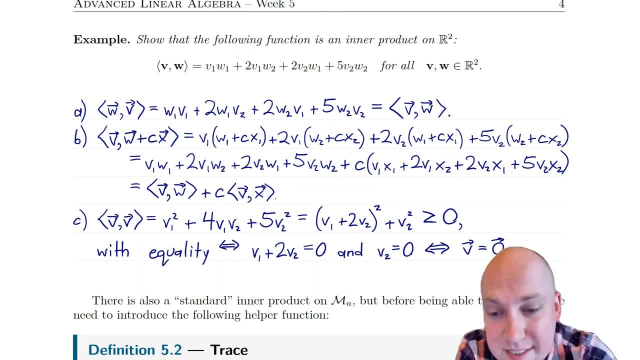 trick is to factor things so that it's a sum of squares. It's this cross term that makes it not obviously bigger than or equal to zero. So factor it into some factor that has this as its cross term when you expand it out. In other words, what I'm going to do is I'm going to say okay. 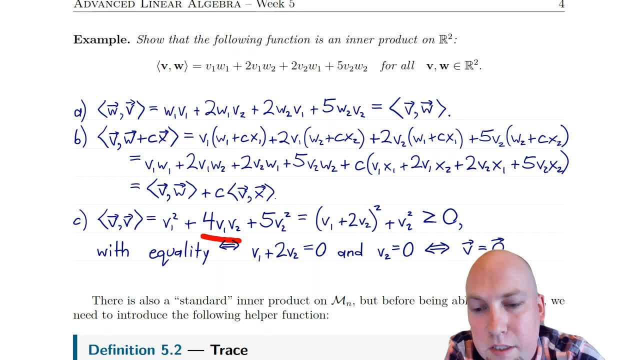 I want some term that when I square it out, I get a V1 squared and I also get this cross term All right, And the sort of binomial that works, the binomial that does the job, is V1 plus 2V2. 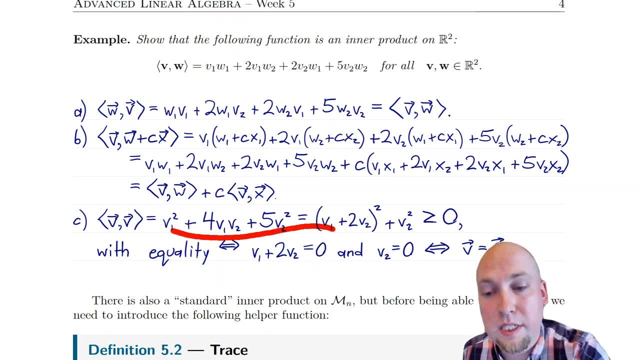 all squared right. Think about what happens if you expand this out. I'm going to get a V1 squared and I'm going to get double this times this. So I'm going to get 4V1V2.. So I'll. 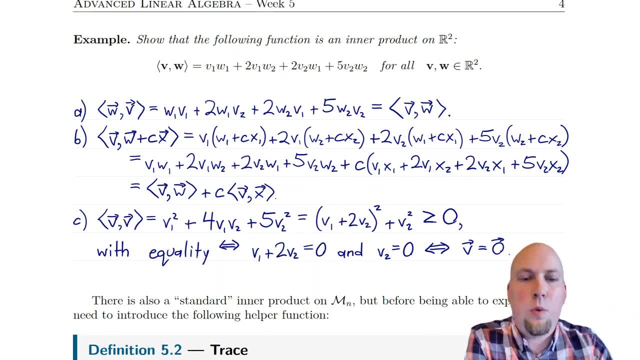 get the cross term All right. The final term isn't quite right, but it turns out that's okay The final term. I'm going to get 4V2 squared. I want 5V2 squared, So just add on another V2 squared. 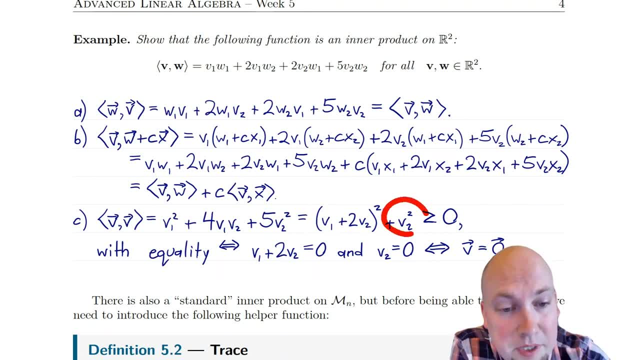 And then this is really good, right, Because I've got something squared plus something squared, Great Squared things are bigger than or equal to zero. So when I add them up, bigger than or equal to zero. Okay, And furthermore, remember you have to check. 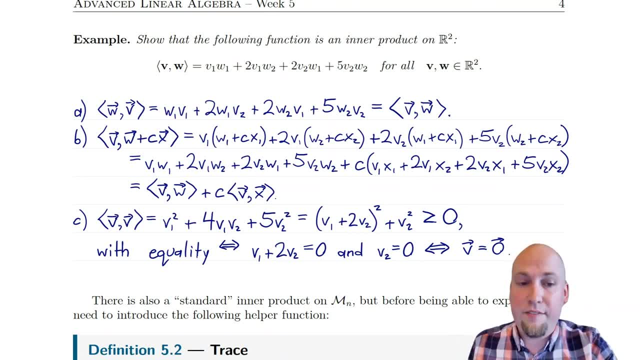 when do I get equality here? Okay, Is the zero vector the only vector that actually gives me equal zero here? Well, the only way that I can get this equal to zero is if both of these terms that I'm squaring and adding up equals zero. So, in other words, V1 plus 2V2 has to equal zero. 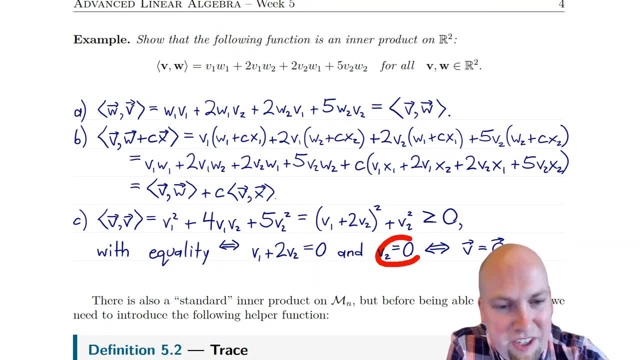 and V2 has to equal zero. But hey, if V2 equals zero, then over here we get V1 equals zero as well. So the only way that it can happen is, yeah, if it's the zero vector. So that weird function, there really is an inner product. It's an ugly one, but it is one. 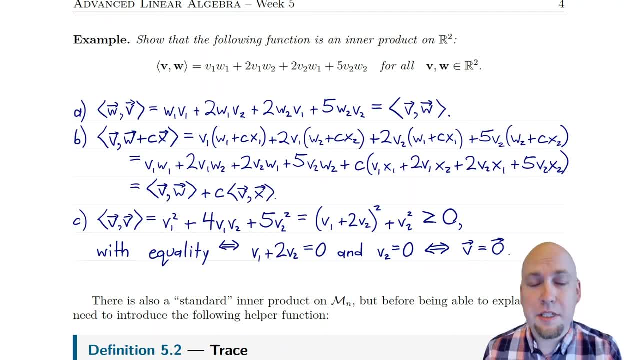 Okay, That will do it for our introduction to inner products. I will see you all next class when we look at the standard inner product on the space of matrices.